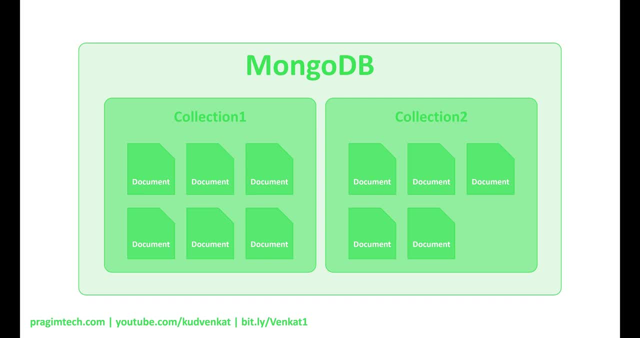 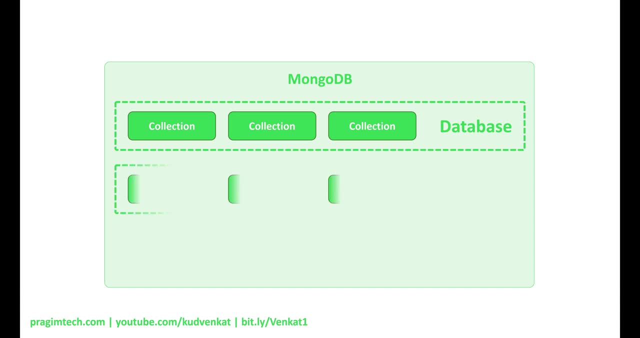 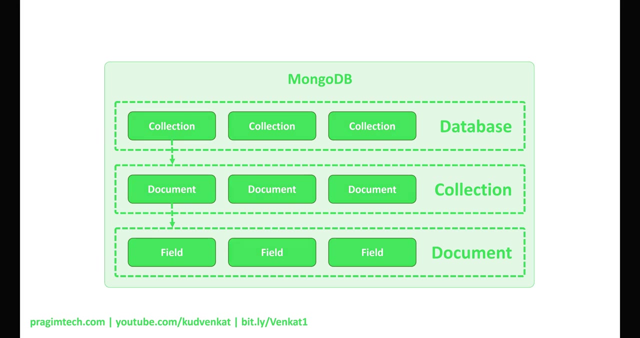 you can think of a collection as a table and documents as table rows. So in MongoDB, a database contains one or more collections. a collection is made up of one or more documents and each document is made up of one or more fields. Now, both in SQL- that is relational- and 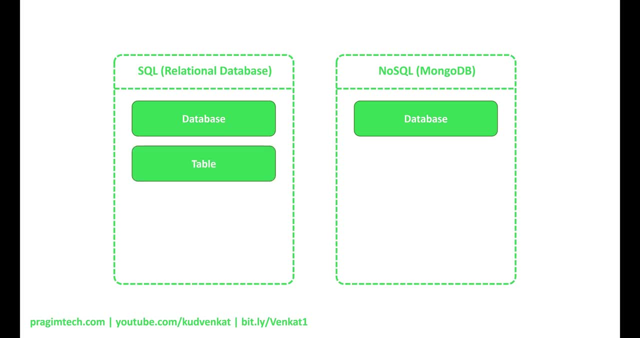 we have tables and in a non-relational world like MongoDB, for example, we have collections. Table rows in SQL world correspond to BSON documents. in MongoDB, BSON is binary JSON. We'll discuss JSON and BSON and the difference between them in just a bit. A column in the SQL world corresponds to 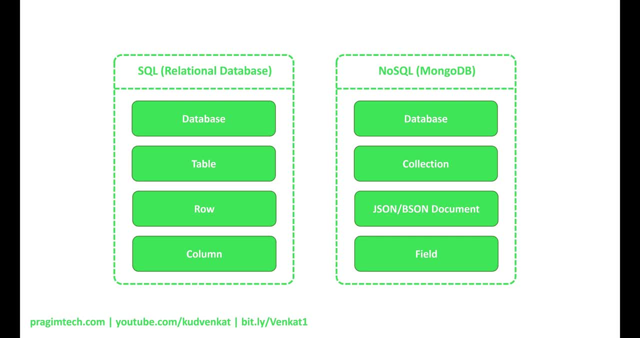 a field in a JSON document. Now it gets a bit easier if we understand these four technical terms: MongoDB, Collection, document, JSON and BSON. So in a nutshell, think of a collection as a table and a document as a table row. Now let's switch gears a bit and understand JSON and BSON At the 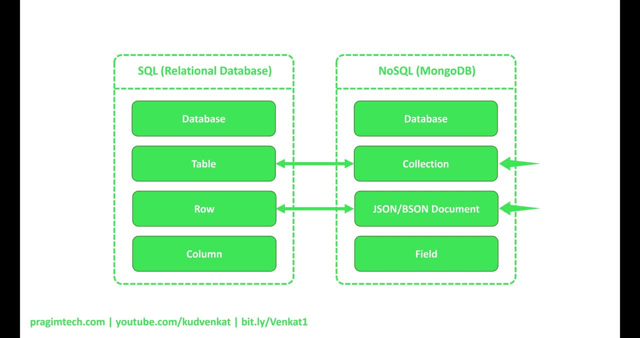 end of the day, MongoDB is a database and we use it to store data. In a relational database like SQL server, data is stored in a table, obviously in rows and columns. In MongoDB we do not have tables. Instead, we have documents. So data in MongoDB is stored in BSON documents. BSON is binary JSON, So 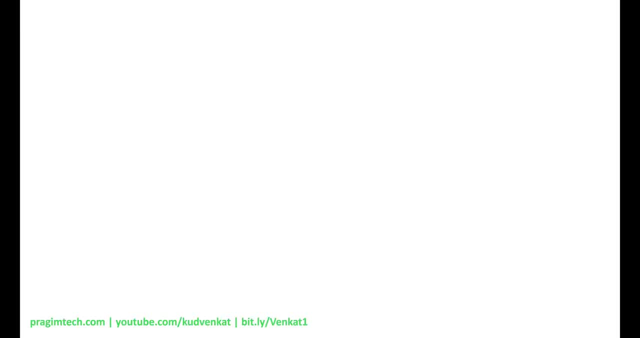 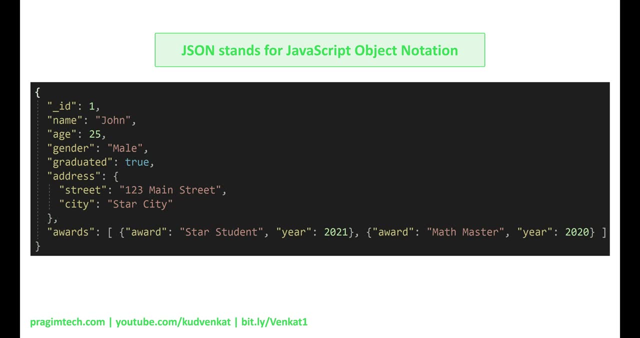 first let's understand what is JSON. The acronym JSON stands for JavaScript Object Notation. In this example, we have student data. JSON format is text-based and both humans and machines can very easily read it. This is the reason it became a very popular format for storing and exchanging. data between software devices. Now let's take a look at the data storage in MongoDB. You can see that JSON is based on BSON. This is the problem that is involved with the data storage in MongoDB. This is the problem that is involved with the data storage in MongoDB. This is the problem that is involved with. 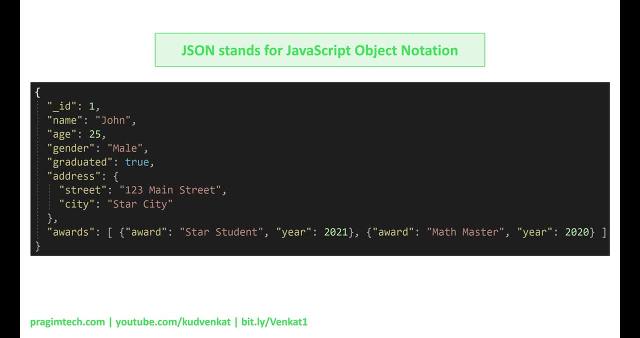 systems. Data in a JSON document is stored in key value pairs. Example name: colon John. A key value pair consists of a field name in double quotes, followed by a colon, followed by a value. Value can be a string, number, boolean or an array. In this example, name field value is a string. age is: 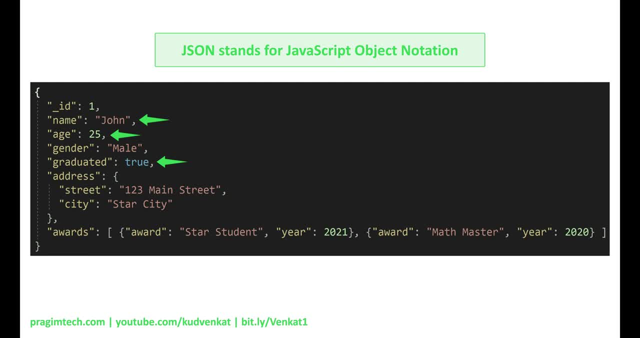 a number. graduated is a boolean value. true or false awards is an array. A field value in a JSON document can also be another nested JSON document. In this example, address field value is another JSON document with its own set of fields and values. So the address is an embedded JSON document. 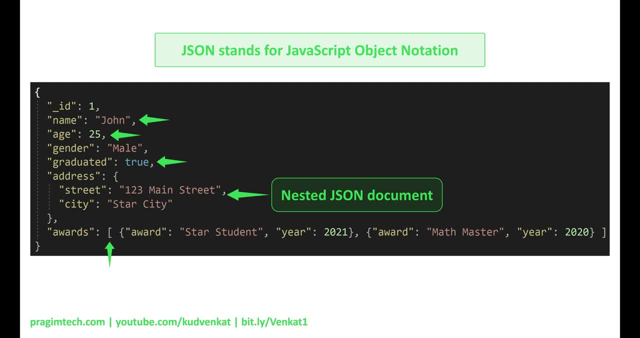 There is a one-to-one relationship between student and address. To model something like this in a relational database, we may have two tables: Students stores students data. Addresses store address data. To retrieve data, we have to join and query both the tables. In mongo we have the entire data in one document. 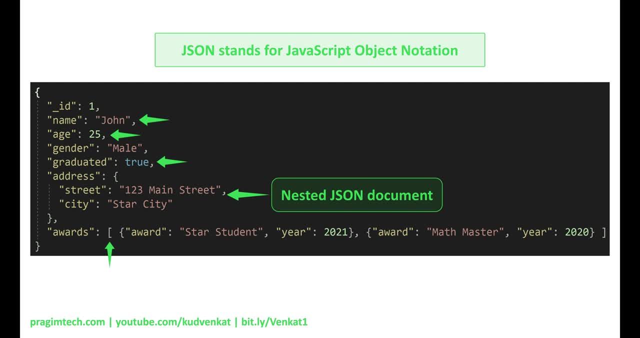 There is obviously no need for expensive join operations. Awards field value is an array. A student may have received zero or more awards, So there's a one-to-many relationship between students and awards. Again, to model something like this in a relational 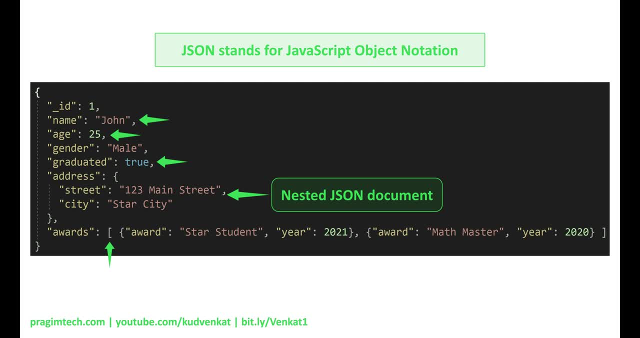 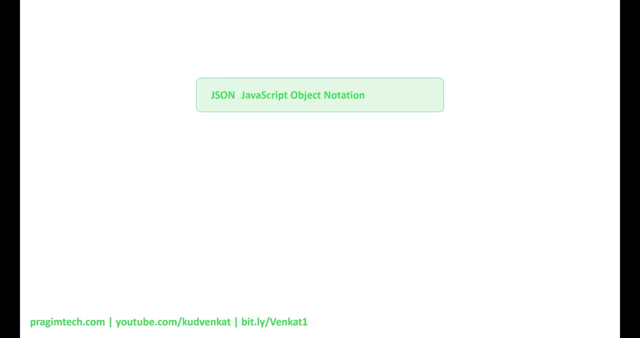 database. we may have two database tables: Students stores- students data- Awards stores. students data stores- awards data. In Mongo we have all the data in one JSON document. Now what's the difference between JSON and BSON? JSON stands for JavaScript Object Notation and BSON stands for Binary. 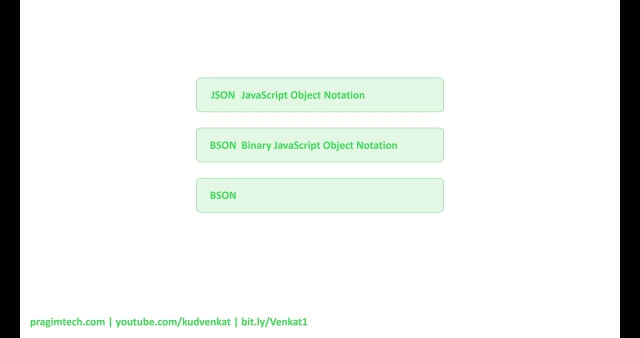 JavaScript Object Notation. Simply put, BSON is binary JSON and it is in this format MongoDB stores data internally on the disk. So, in a nutshell, BSON is the serialization format used in MongoDB. At this point you might be wondering: we already have JSON. why did MongoDB invent BSON? 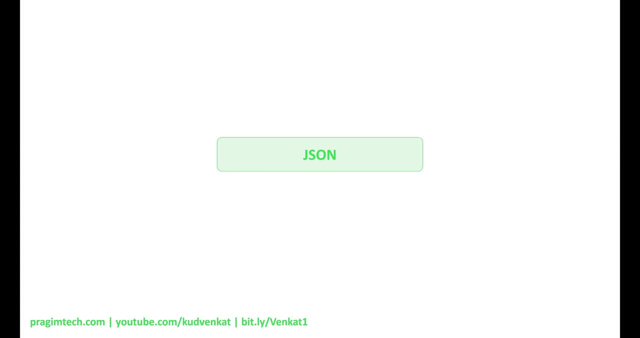 Well, JSON only supports a limited number of basic data types: String, Boolean Number, Array. Also, JSON is a text-based format and parsing JSON text is very slow. We want database engines to be fast. we don't want text parsing to slow it down. hence MongoDB invented BSON. The following are the three: 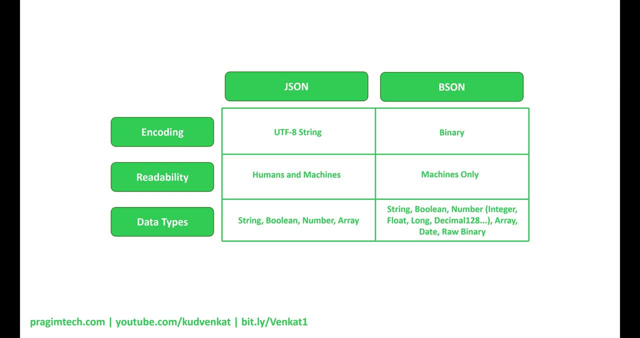 things that we need to know about BSON. First, we need to know how to use BSON in MongoDB. Second, we need to know how to use BSON in MongoDB. Third, we need to know how to use BSON in MongoDB. Fourth, we need to know how to use BSON in MongoDB. At this point you might be wondering: should I now? 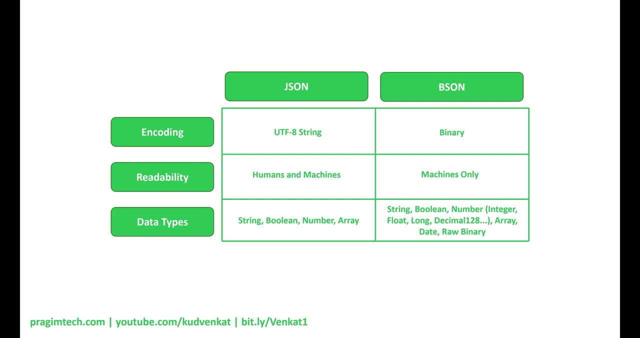 learn this new binary BSON format? Well, no, As developers, we still use JSON format, and MongoDB takes care of converting it to BSON and saving it on the disk In your JSON documents. if required, use the additional data types provided by BSON. We don't have to worry about. 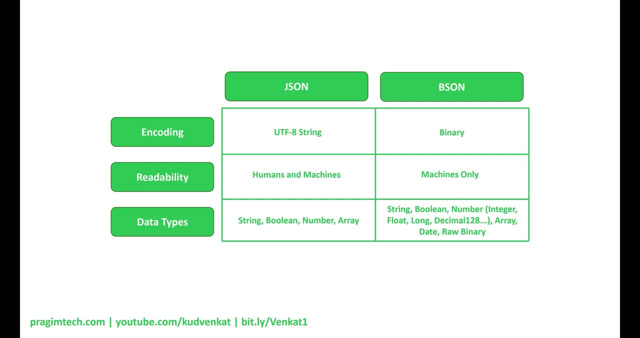 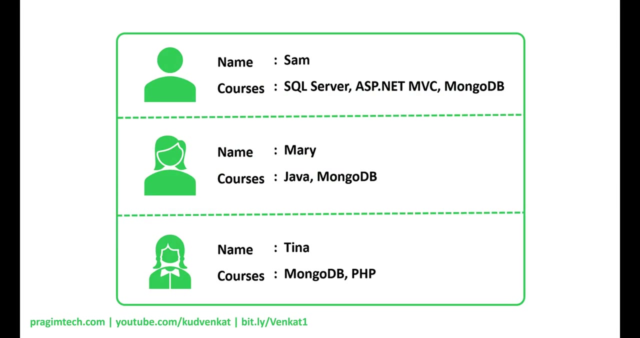 the internal BSON format. it's all taken care of by MongoDB. Remember, BSON is a binary representation of JSON and it contains more data types than JSON, So you can think of BSON as a superset of JSON. Now let's take a look at a very simple but a real 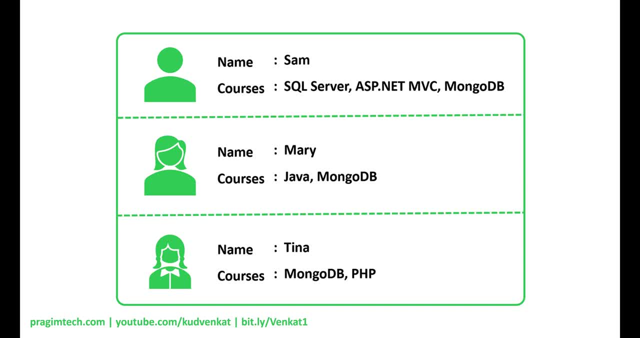 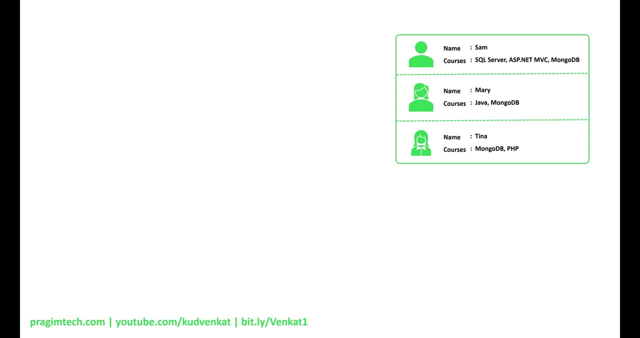 world use case. Let's say we are developing an application for a training institute and we have a page that displays student names and the courses they have enrolled in on a web page. as you can see right here, To model something like this in a relational database world like SQL server or Oracle, we typically create three. 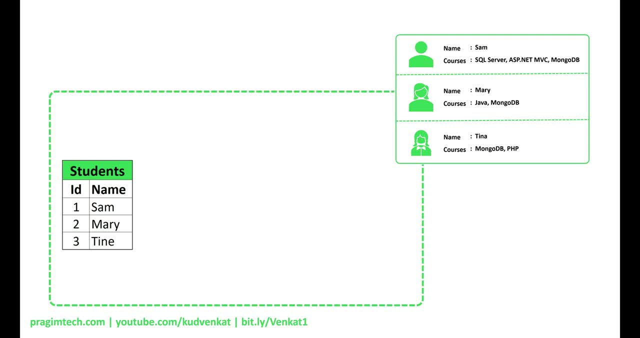 tables: Students: stores the details of students, like ID and name. Courses: stores: the course details, like course ID and name. Student courses: there is a many-to-many relationship between students and course tables, meaning a student can enroll in multiple, that is, many- courses. 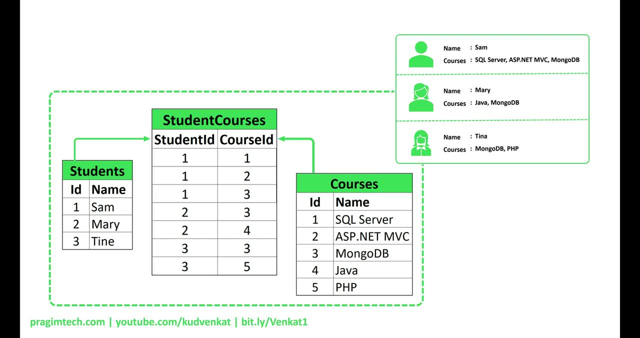 Similarly, a given course can have multiple students enrolled. So this is a very simple way to model a course. Now let's take a look at the BSON database. Let's take a look at the BSON database. So let's take a look at the BSON database. So 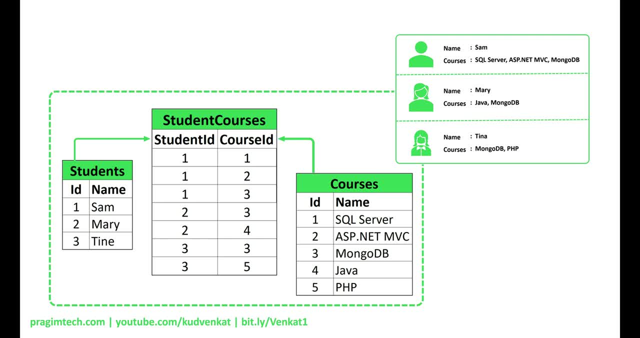 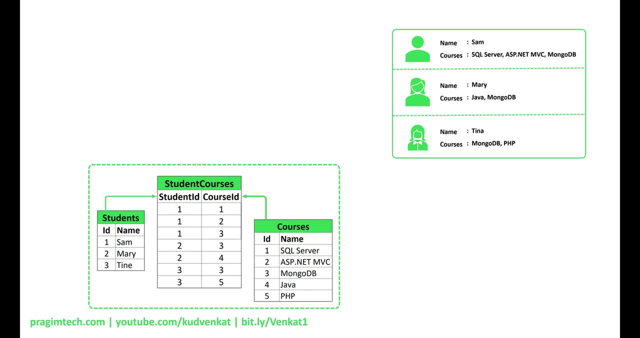 this is the table that links students and courses, basically the bridge table for many-to-many relationship between students and courses. On the application side, to be able to display this database data, we may have a class that looks like the following: This is a very 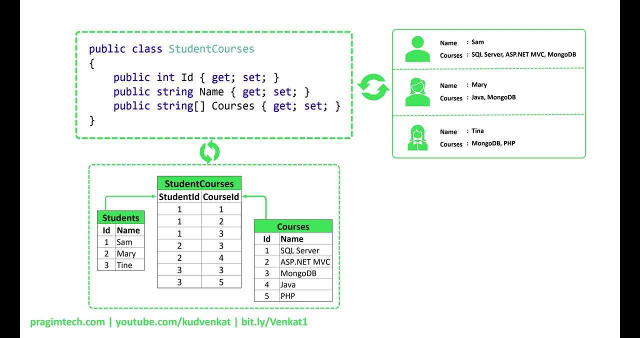 very simple example here: In the real world, in our application layer we may use object-oriented programming concepts like inheritance, polymorphism etc. between classes, which makes it even more difficult and a painful exercise to map our application layer objects to database. 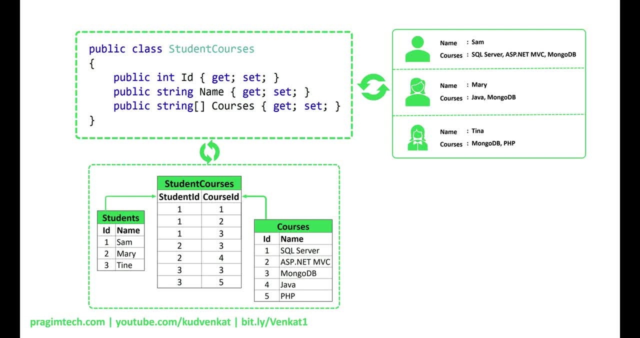 tables and rows. So the point that I'm trying to get across is there is a lot of misalignment between application classes and database tables. Simply put, our application objects are not tables and rows. Now, to fill this gap and misalignment, we may write a custom mapping layer or use ORMs. 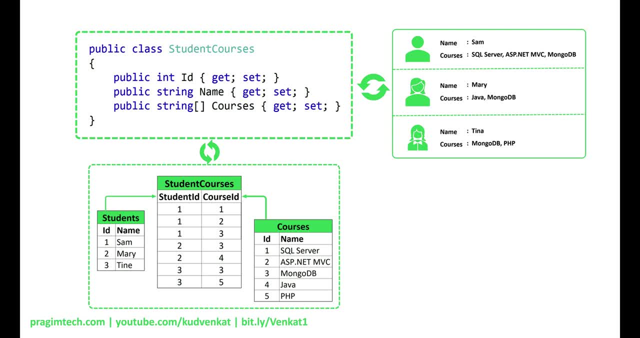 that is, Object Relational Mappers, like Entity Framework, for example. As software engineers, we want to reduce all this complexity and use of additional softwares. Instead, we want a database that is easy to use with our application code. Now let's see how this. 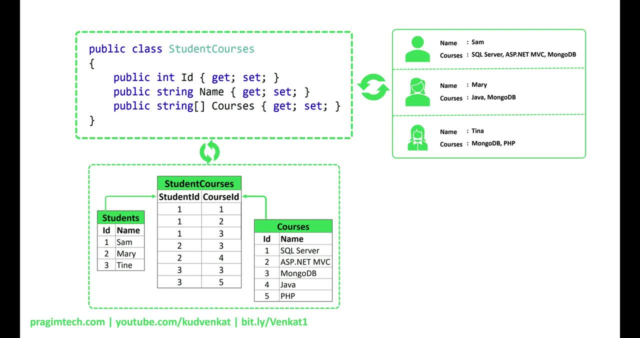 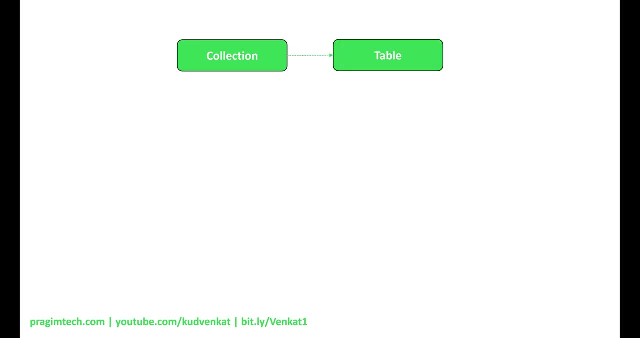 same data may be stored in a non-relational database like MongoDB, As we have already discussed. in Mongo we do not have tables and rows. Instead, we have collections and documents. You can think of a collection in MongoDB as a table in a relational database and 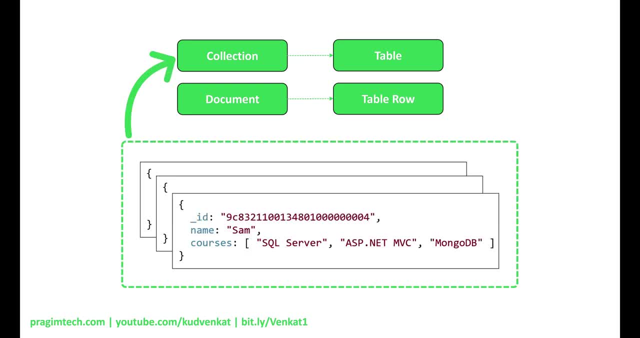 a document as a table row. In this example, we have one collection. The name of the collection is StudentCourses. In this collection we have three documents. So, just like how a table is a container for rows, a collection is a container for documents. It is the document that physically 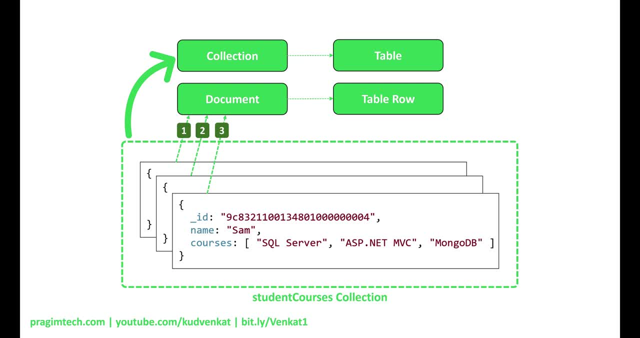 stores data. The data is in BSON format, So the documents are also called BSON documents. If you are wondering what is BSON, well, it's binary JSON. MongoDB stores data on the disk in BSON format, The same Students and Courses data that we have across three tables in. 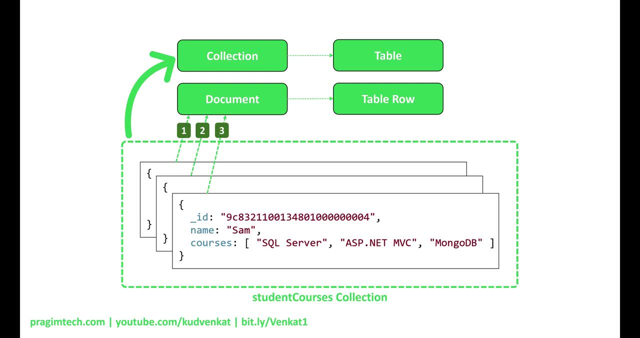 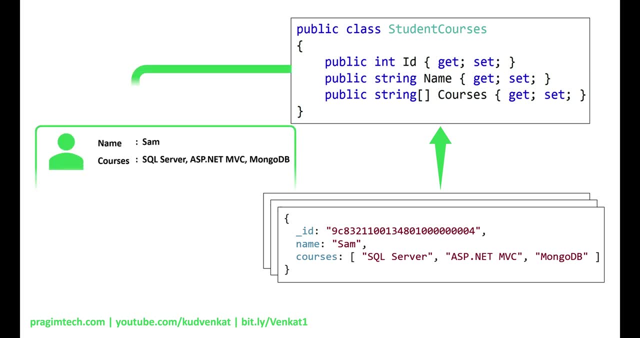 a relational database can be stored in a single collection in Mongo, as shown right here. For any application. this data is very easy to work with. No complex joins and mapping layers are required. Our application code will be much cleaner, simpler and easier to maintain. So does this mean we cannot define relationships between documents? 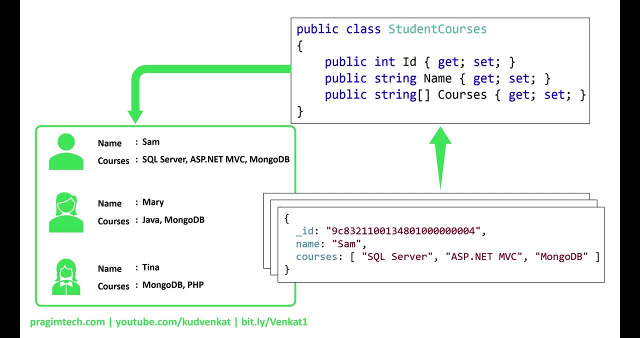 in a non-relational database like MongoDB. Well, we can define relationships between documents in MongoDB, but these are usually capped to an absolute minimum. In most cases, we embed JSON documents inside another document. The obvious benefit of this approach is we have 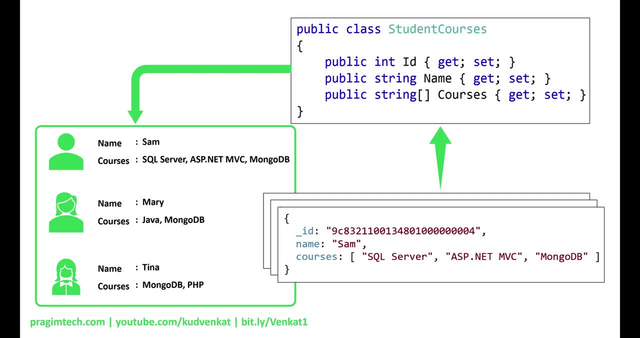 all the data we need in one place and there is no need to traverse multiple related documents. Here's the important bit. We can define relationships or references in MongoDB. We can even completely normalize schema in MongoDB, just like a relational database. But the question is if you want to normalize and use a non-relational database like a relational. 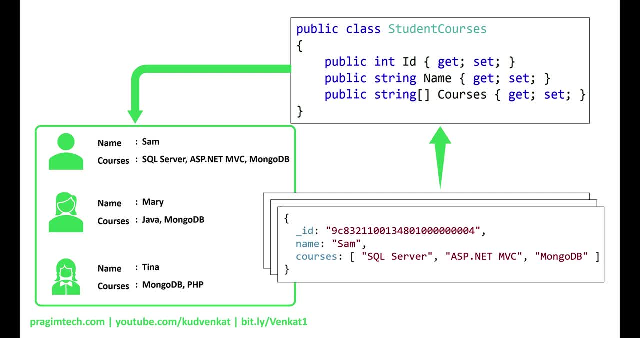 database. why use a non-relational database? Use a relational database like SQL Server or Oracle. This nicely leads us to another common question we may have: when to use a relational database like SQL Server over a non-relational database like MongoDB, and vice versa. Well, relational databases are still the best choice if the data is predictable in 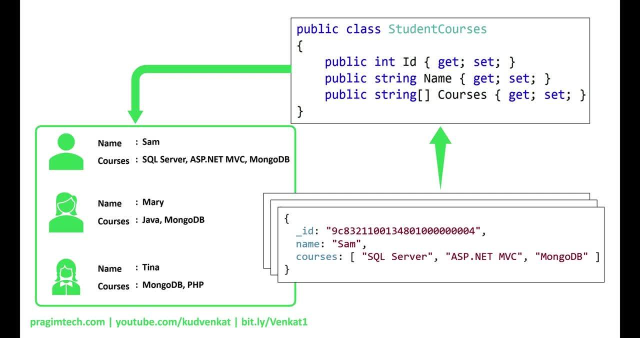 terms of structure, size and frequency of access. Also, if relationships between entities are important, again relational databases are the best choice. Normalization in a relational database reduces the size of the data on disk by limiting duplicate data and anomalies In a non-relational. 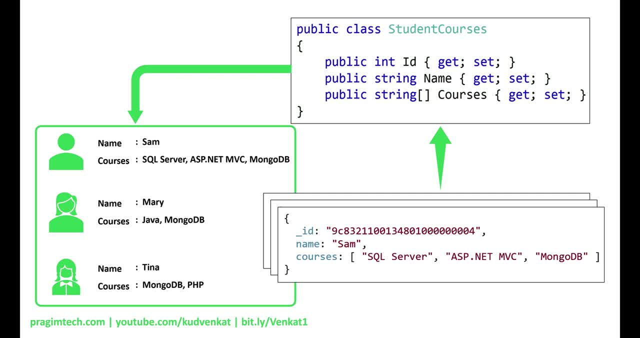 database documents are embedded within documents, which helps keep data that will be accessed together in the same place. But if this isn't right for your needs, use a relational database, For example, if you have a very large data set with complex structure and relationships. 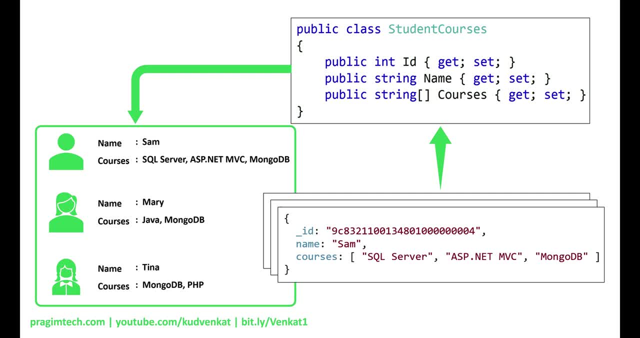 embedding might not create clear enough relationships. Finally, relational databases have been around for a very, very long time, which means there is wide support available, from tools to integration with data from other systems. On the other hand, if you want a flexible schema for the data, that is, in terms of shape or size, or if it needs to be open to change, 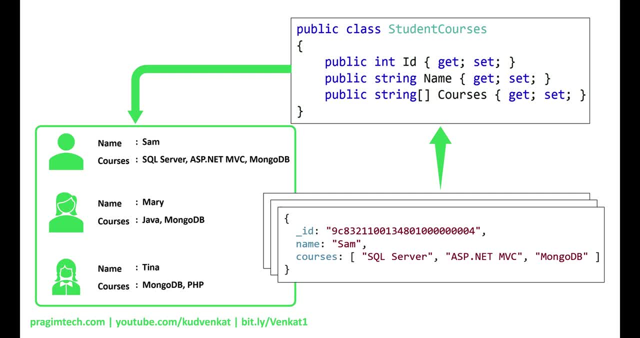 in the future, then a non-relational database is the answer. Non-relational databases have been designed from the ground up for the cloud, which makes them naturally good for horizontal scaling, where lots of small servers can be spun up to handle increased load. Now, what is NoSQL? Lots of people use these two terms. 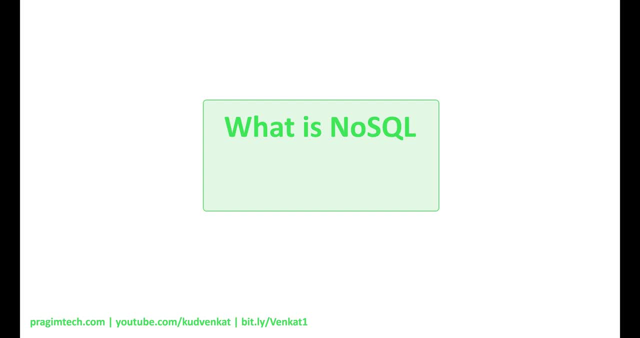 NoSQL database and non-relational database interchangeably. A non-relational database like MongoDB is more than a NoSQL database. So what does NoSQL stand for? Well, when we hear this term NoSQL, we think NoSQL means there is NoSQL. This is not true. The term NoSQL stands for not. 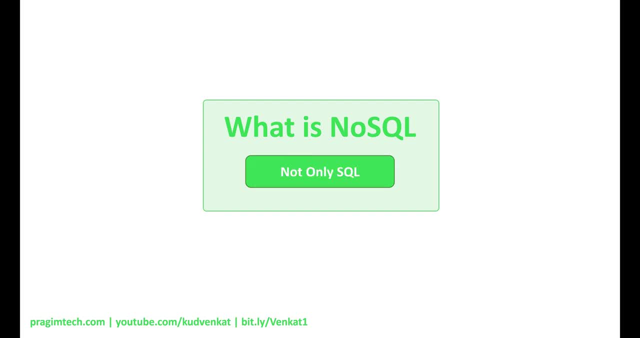 only SQL and it means a non-relational database is a non-tabular database and stores data differently than relational tables. For example, in a relational database like SQL Server or Oracle, data is stored in tables, whereas in a non-relational database like MongoDB, data is. 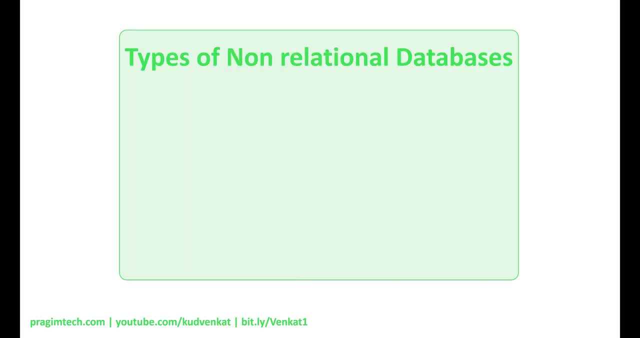 stored in JSON documents. There are different types of non-relational databases. Document database, As the name implies, data is stored in documents, For example, in JSON documents. Examples of document databases are MongoDB and CouchDB. Key-value database: It stores data as 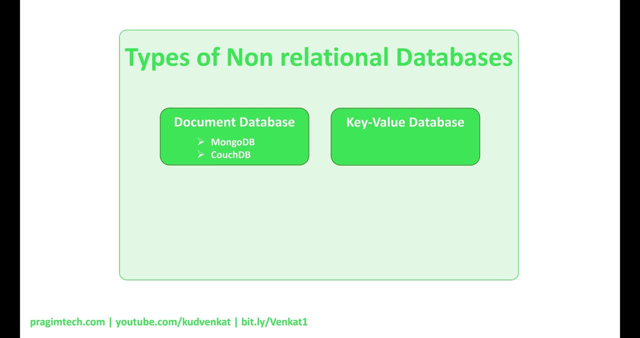 a collection of key-value pairs in which a key is used as a unique identifier. Both keys and values can be anything ranging from simple objects to complex compound objects. Examples are DynamoDB and Redis Wide column store. It's similar to a relational database in the sense it stores data. 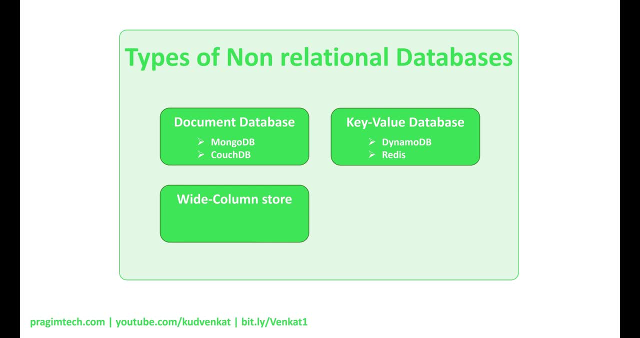 in rows and columns. However, the columns are dynamic and each row does not have to have same columns. Examples are HBase and Cassandra. Finally, graph database. It is used to store and navigate to the kind and number of relationships. It's heavily used in fraud detection and social. 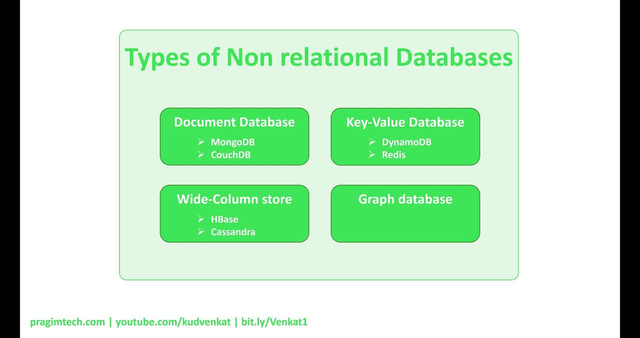 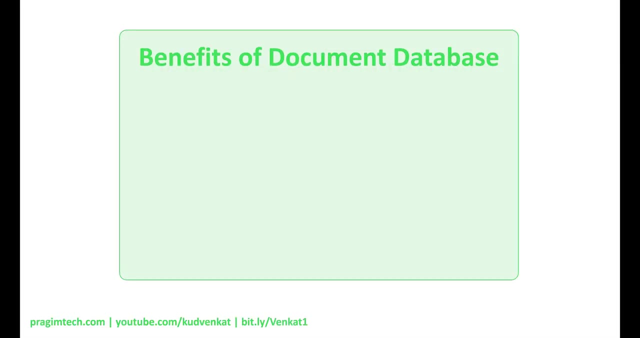 networking, It is easy to create relationships between data entities and quickly query these relationships. For example, you can find out who the friends of friends of a particular person are. Examples: DGraph and OrientDB. Now let's focus on the benefits of using a document database It has. 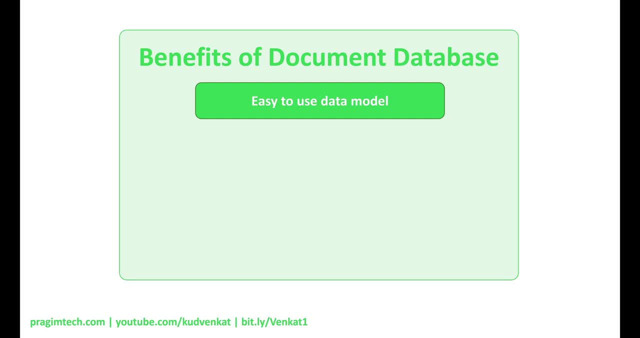 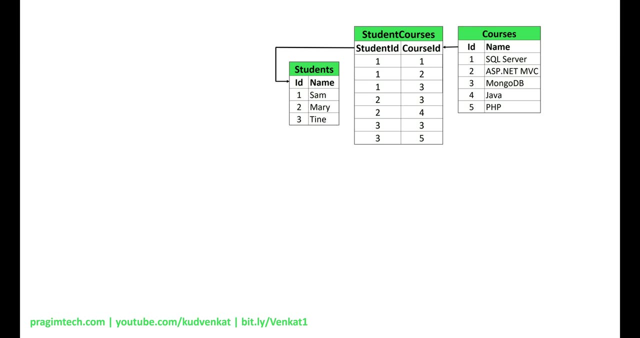 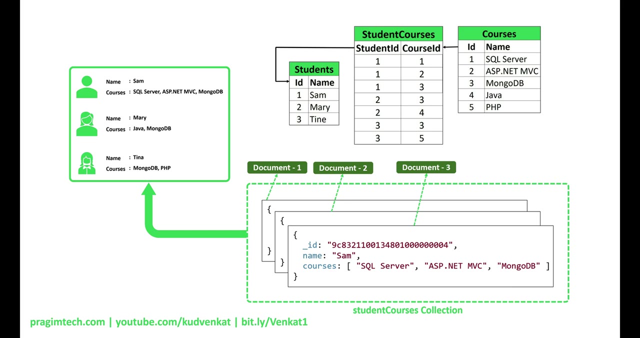 a database like MongoDB, We do not have tables and rows. Instead, we have collections and documents. The data that we typically store across many, many relational database tables can be stored in a single collection For an application. this data is very easy to work, with No complex joins and 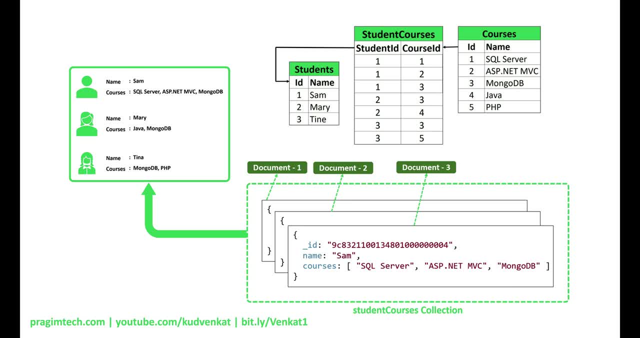 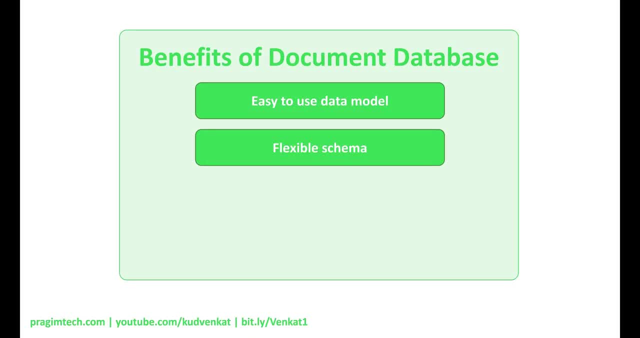 mapping layers are required, Our application code will be much cleaner, simpler and easier to maintain. Flexible schema is another benefit. JSON documents that actually store data have a flexible schema, which means it's perfectly okay and normal for two documents to have different fields. In this example, we have two documents with student data, Both the 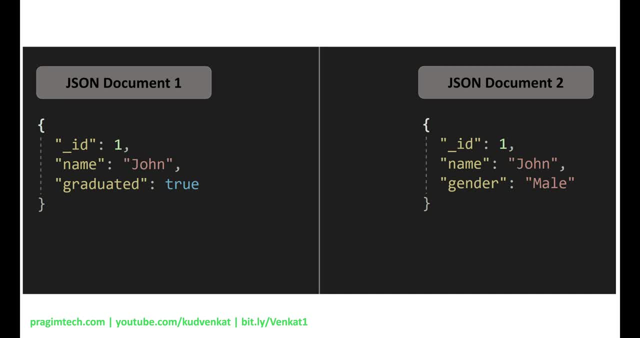 documents have id and name fields. In the first document we have graduated boolean field, whereas in the second document, instead of graduated, we have a string gender field. So the point is, document schema in Mongo is dynamic and self-describing Every document. 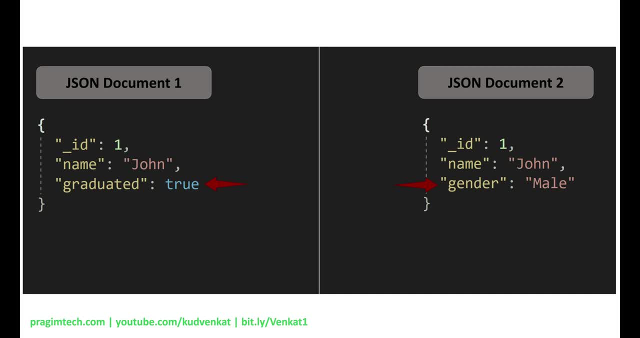 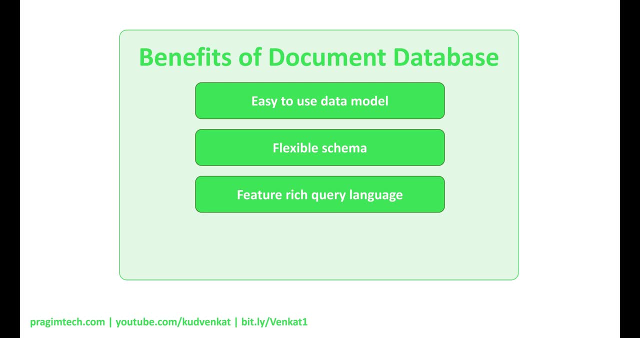 that we save in Mongo can be as flat and simple or as complex as our application requires. MongoDB Query Language is based on JavaScript and very easy to learn. When querying data, you have a wide range of options, operators, expressions and filters. Data is very easy to query. 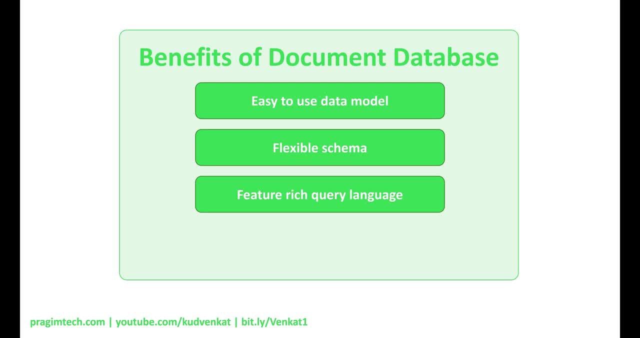 and you rarely need joins or transactions. The MongoDB Query Language is a full-featured, powerful language that allows you to query deep into documents and even use the aggregation framework to perform complex analytics with just a few lines. Indexing is also supported, which means documents. 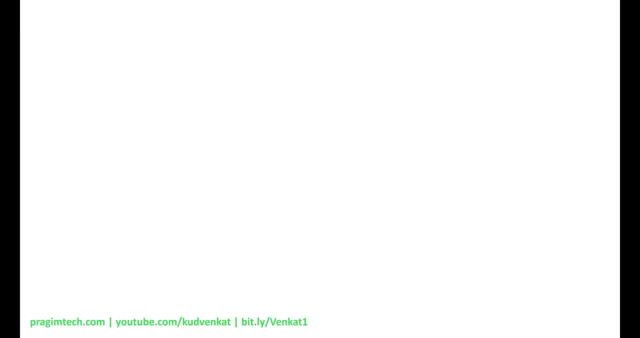 can be retrieved quickly. Most relational or SQL databases allow only vertical scaling, which is also commonly called scaling up. Vertical scaling involves adding more resources like memory storage etc, to the existing database server. Vertical scaling has an upper limit beyond which you cannot just add more CPU memory etc. There is also downtime involved. You have 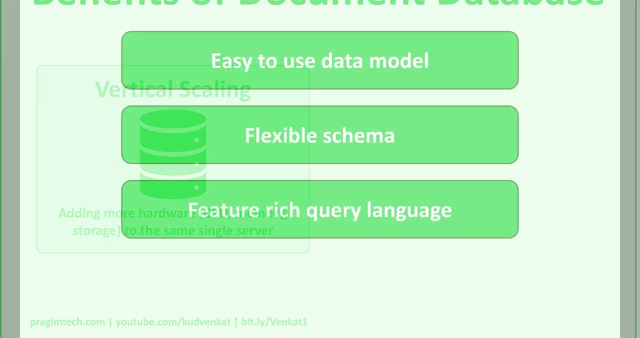 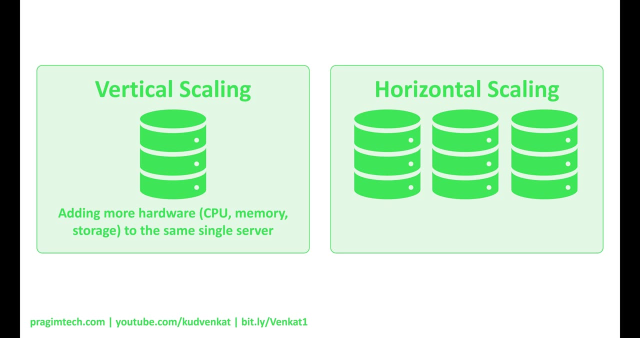 to shut the database server down to add more hardware. MongoDB, on the other hand, supports horizontal scaling, which is also commonly called scaling out. In horizontal scaling, data is partitioned and distributed across many servers, So, in simple terms, scaling horizontally means. 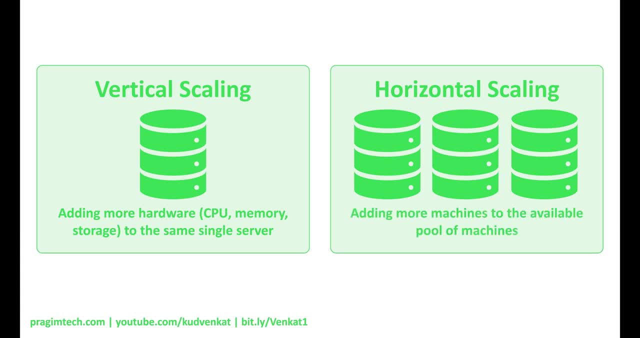 adding more servers to the already existing pool of servers. This means you're not limited to the capacity of a single server. There's no need to turn off existing servers to add a new server to the pool. So there's no downtime as well. 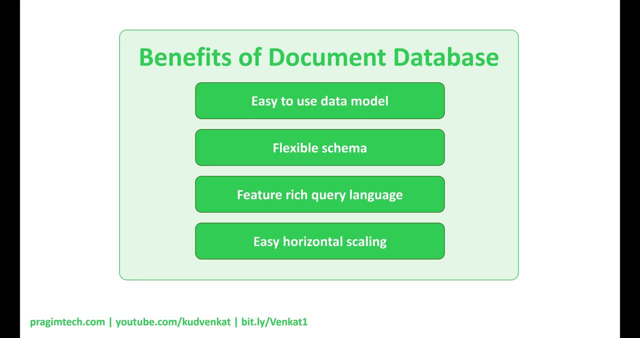 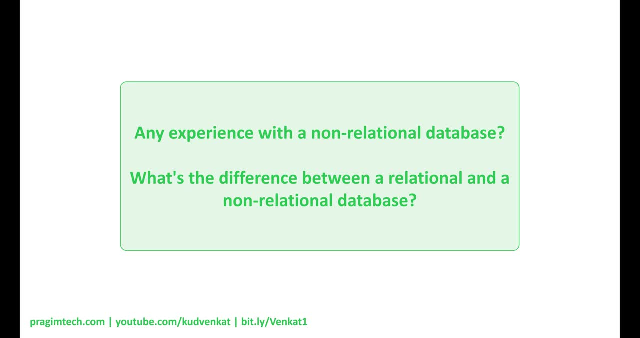 So non-relational databases like MongoDB have become very popular. The following is one of the common questions asked these days in a software engineer interview: Have you got any experience with a non-relational database? What's the difference between a relational and a?